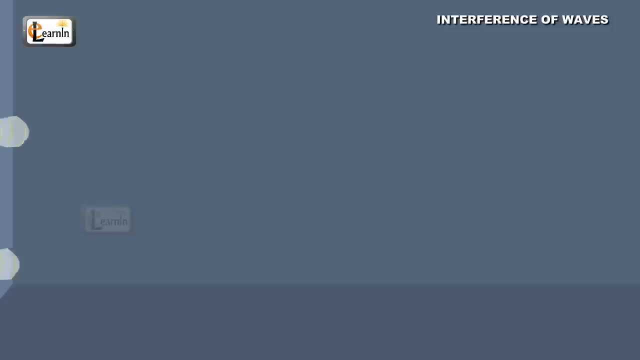 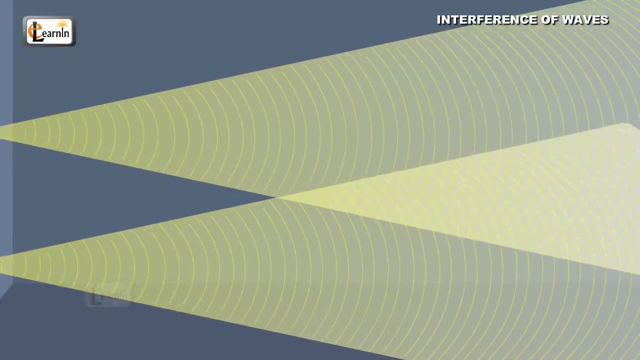 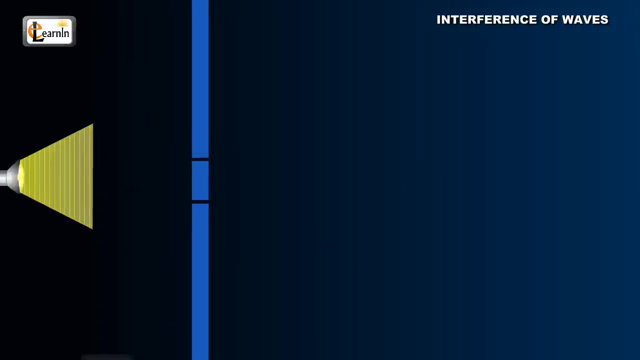 only be explained by the wave theory of light. We know that two or more wave motions travel in space at the same time. Sometimes these two wave motions combine and some physical effects take place. Interference is one such physical effect. When two or more waves cross. 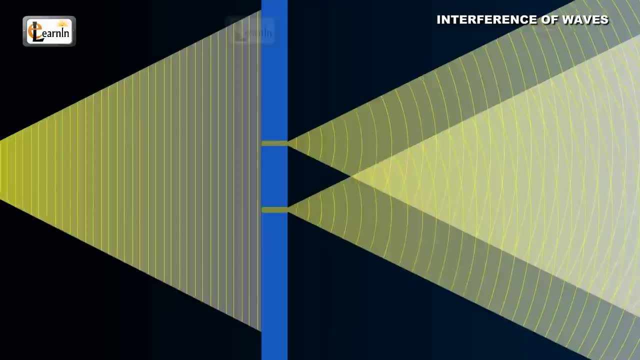 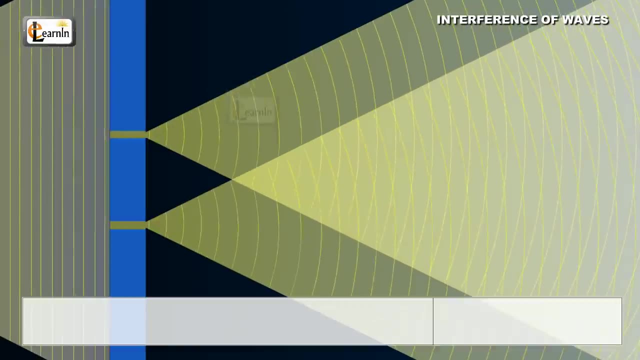 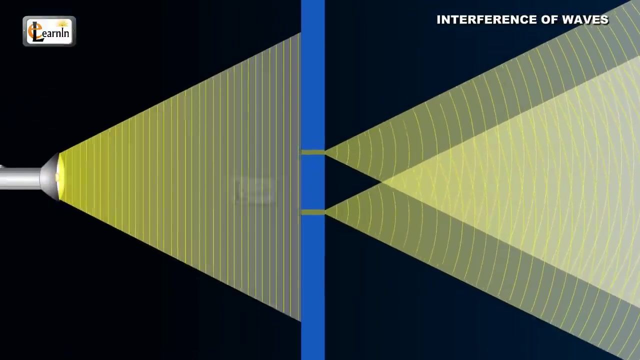 each other in the same medium. they both interfere and an accident takes place. This accident is known as the interference of waves. Interference is the combined effects of the disturbance caused by the each individual wave at the same place, at the same time. This effect can be understood from the principle of superposition of waves. 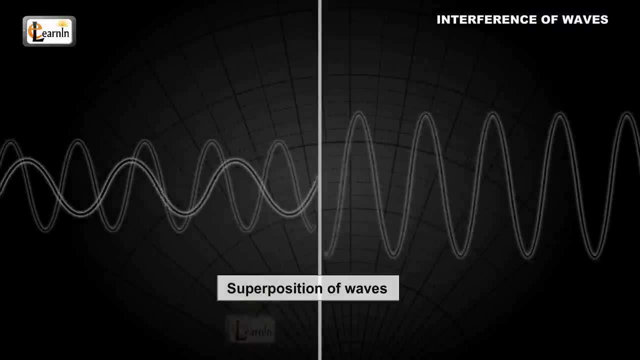 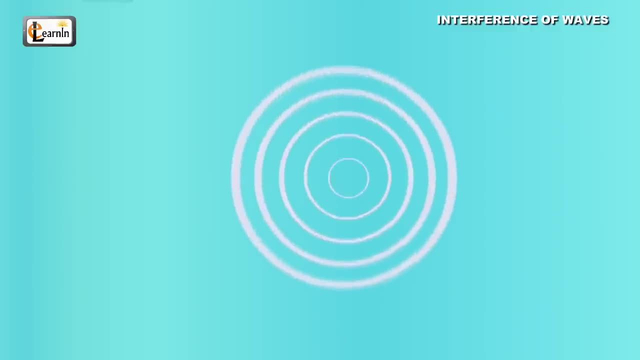 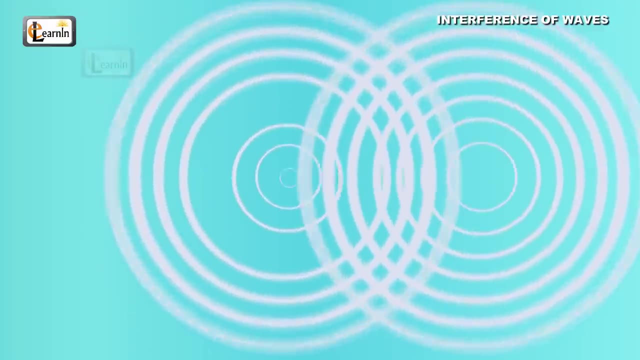 To understand this concept of the superposition, let's understand some of the examples. When we drop a pin in a tank, we see some circular waves. When another pin is dropped, we see some more waves. These waves travel in the same tank and at one time or another they 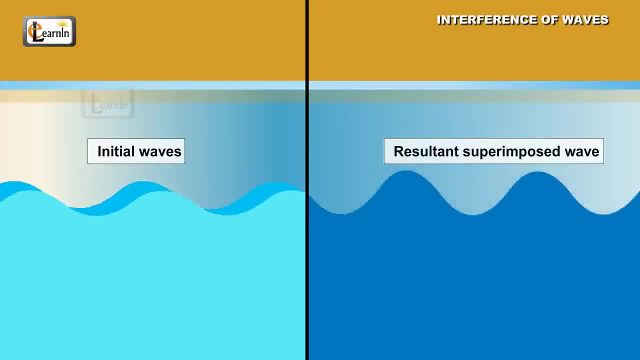 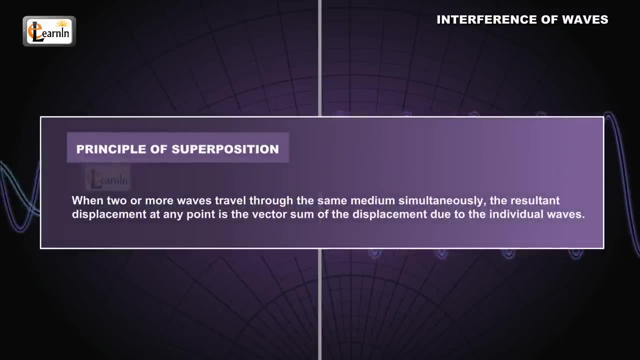 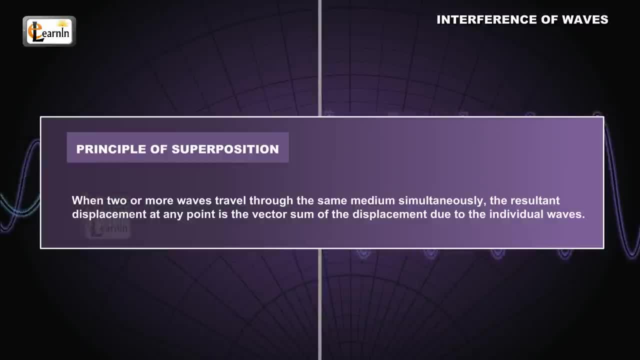 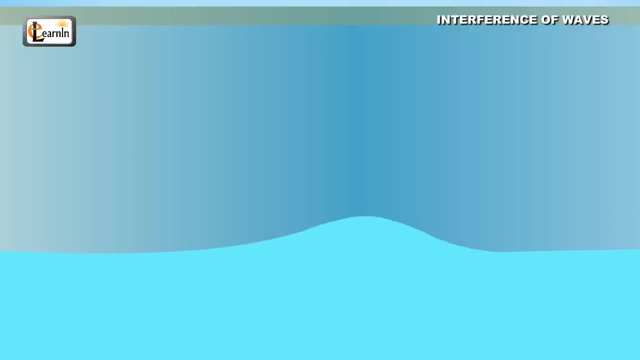 the principle of superpositions of waves states that when two or more waves traveling through the same medium simultaneously, the resultant displacement at any point is the vector sum of the displacement due to theывidual waves. In our case, the pin is dropped in a ripple tank with two pins. If is the displacement caused at a point due to the first source? 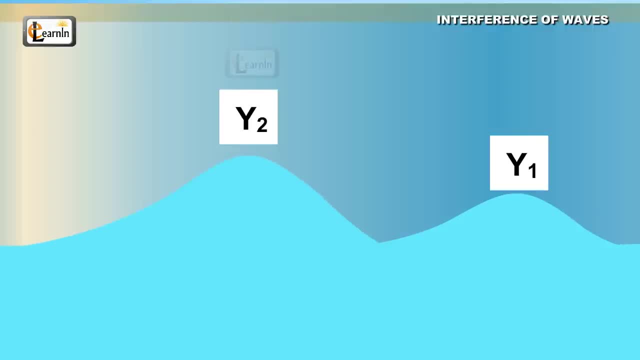 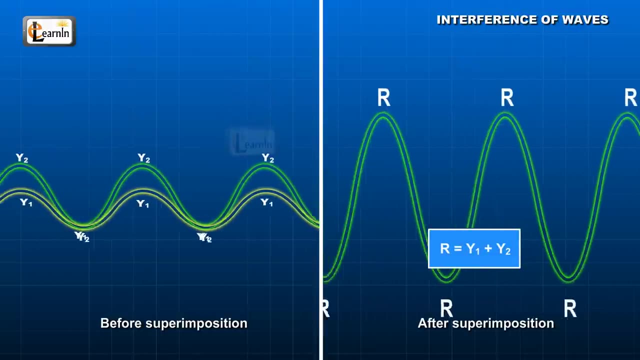 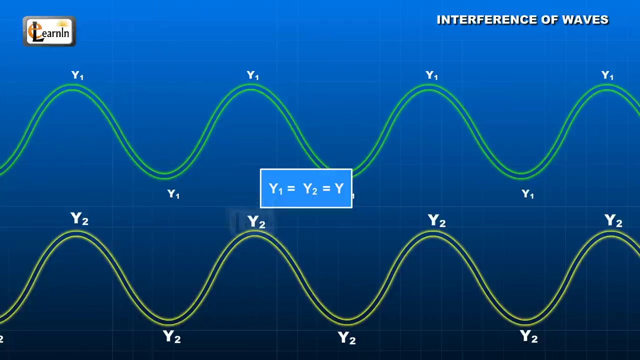 and y2 is the displacement caused by the second source, then the overall displacement r at the point of interference would be given by r equals y1 plus y2.. When both sources have the same amplitude then y1 and y2 would be equal to y. When y1 is due the crest or tro. 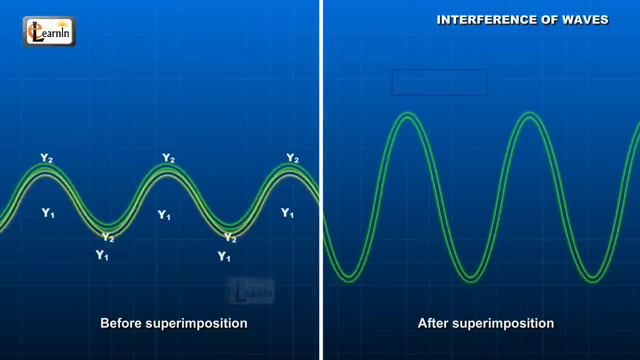 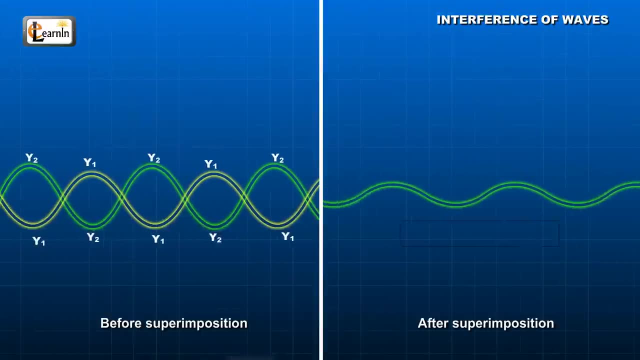 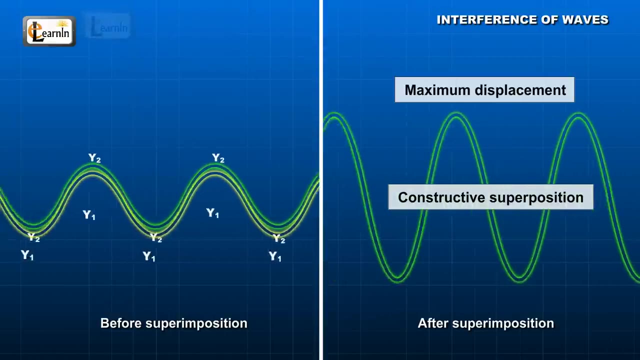 and y2 is also due a crest or tro, the resultant would be the maximum, And when y1 is due to a crest and y2 is due to a tro, or vice versa, the displacement would be minimum. When maximum displacement takes place, it's called constructive superposition.